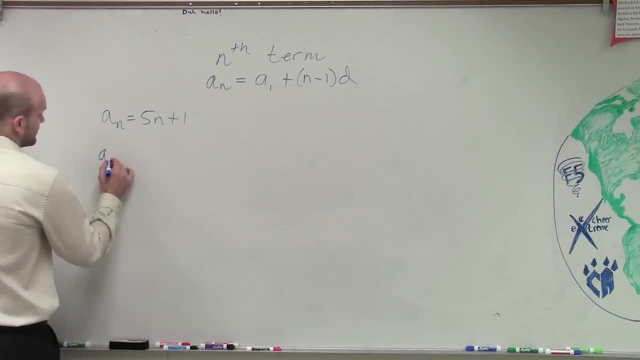 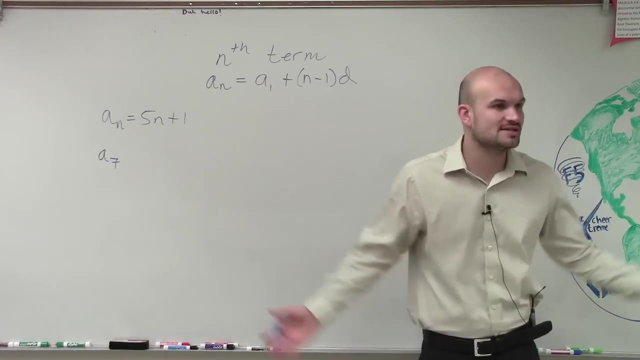 But then there's also a couple questions where I said: hey, what is a of 7, right? Without even going in order of what's the first four terms, I said, hey, what's the 7th term, Or what's the 25th term? Right, Whatever. 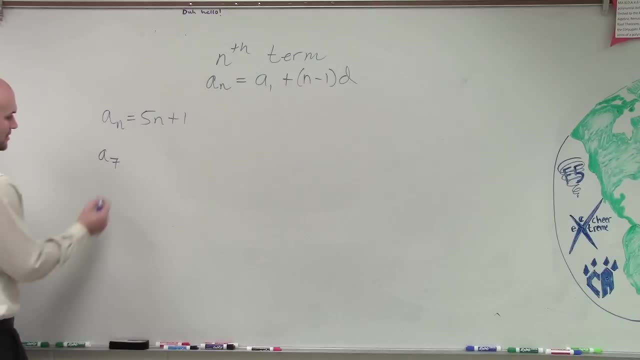 So what you had to do was then plug in whatever number I wanted to. If I said what's the a of 10th term, right, Then you just plug in that number, your term, to find that value, Right? So whatever term I want to find, I could just plug it into my sequence. 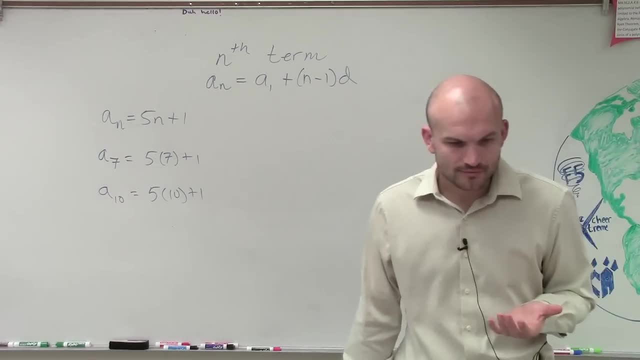 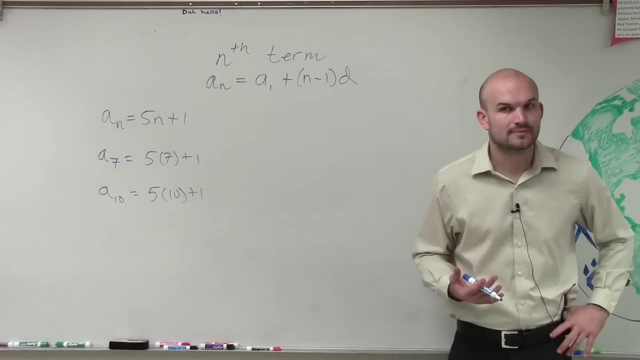 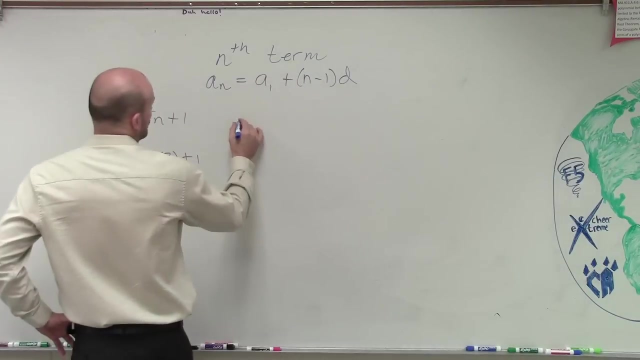 Now what comes up to this is, what happens is, let's say, we're given some information, but we're not given the rule. All right. So let's say we're given some information, but one thing we know is, let's say, I want to find, let's say I know that the difference of an arithmetic sequence is 2.. 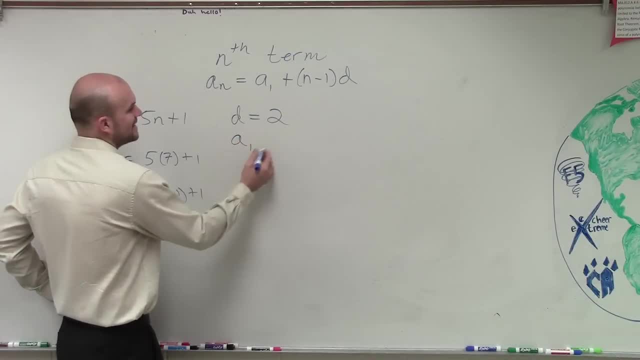 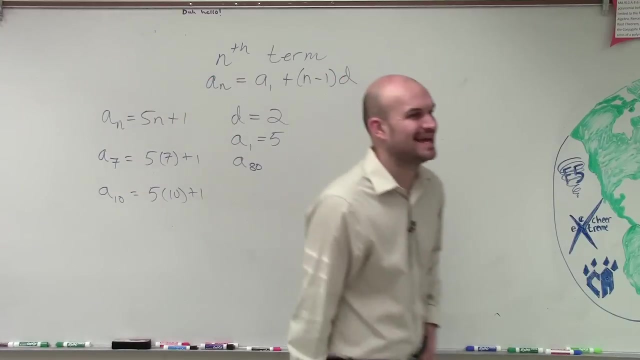 All right, But- and the only thing I know is a sub 1 starts at 5.. Right, And I want to figure out a of 80.. Okay, And I want to figure out the 80th term, Yeah. 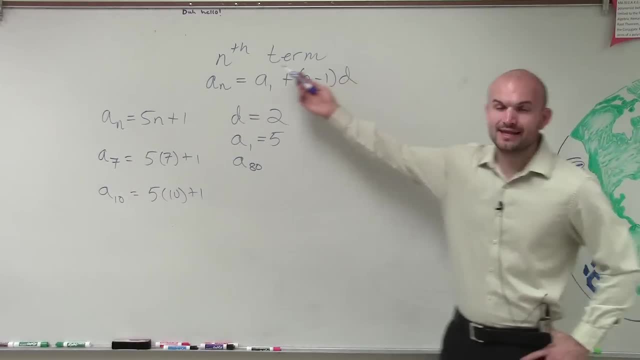 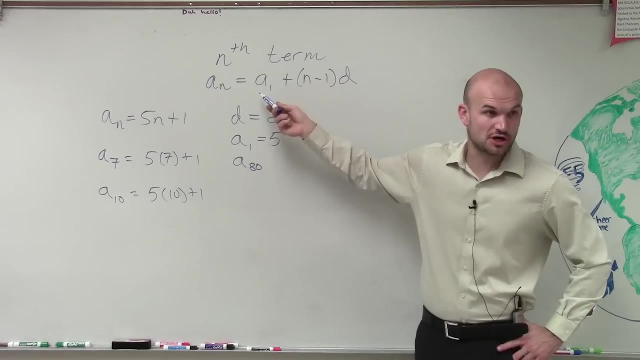 Well, let's see what we have here. Okay, So what the nth term formula says is: whatever your term that you want to find, if you don't know what your rule is, that's going to be equal to the first term. 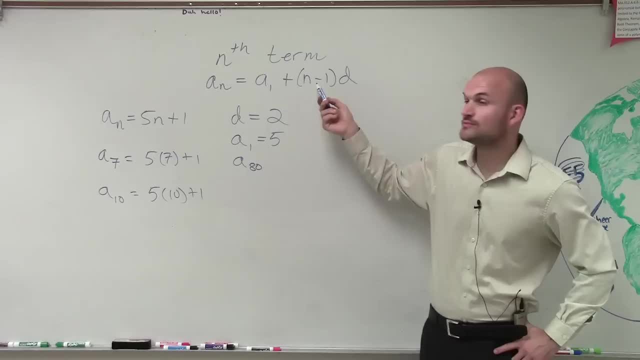 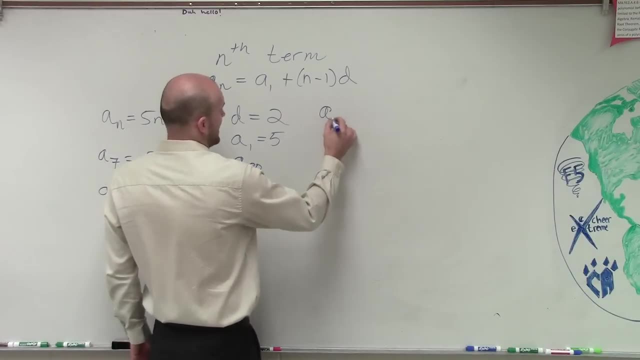 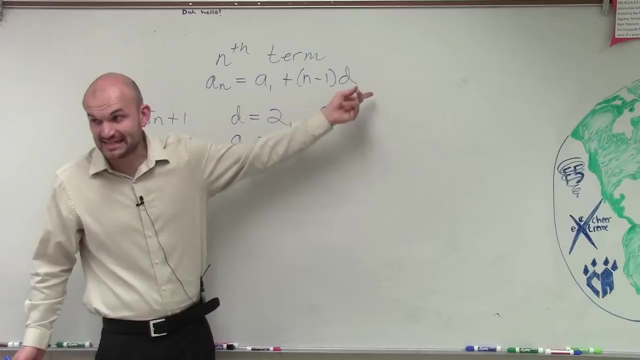 plus your term that you're trying to find minus 1, times the difference. So in this case, which is the example I'm just kind of making up, if I want to find a of 80, right, I want to find the 80th term of a sequence that has a distance of d, right. 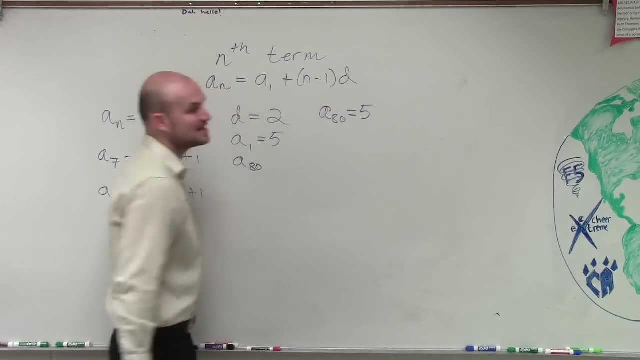 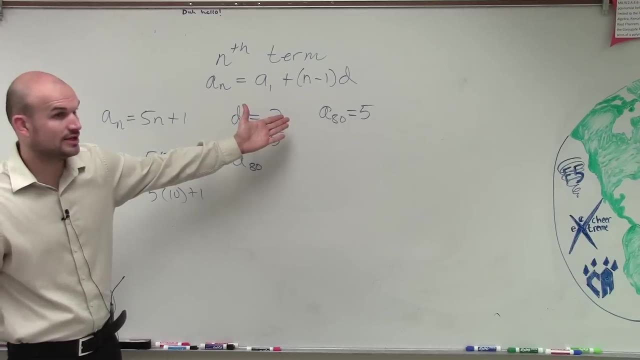 That starts at 1, or, I'm sorry, it starts at 5.. And each term has a difference of 2.. So it's important for us to be able to figure out the difference Right. We don't need to know the rule. 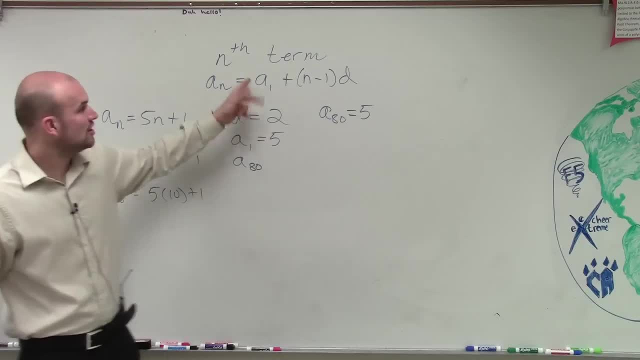 But if we know what the difference is and we know where it starts, we can find the 80th term Right. See how these are kind of different Here. we know the rule. Once you know the rule, you're golden. 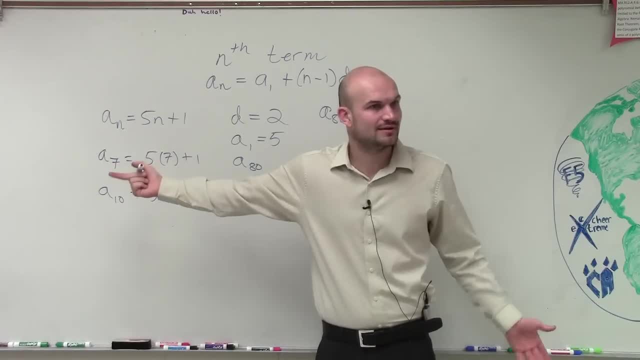 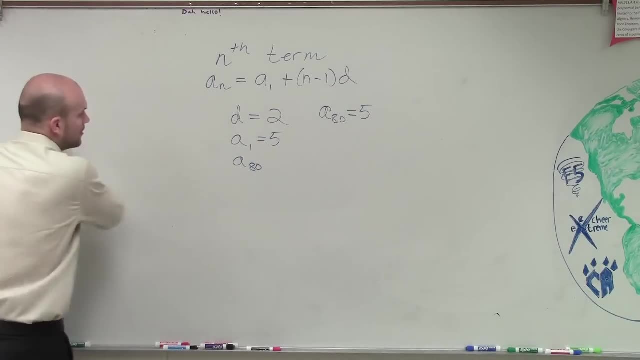 Right, You just plug in that term. You plug in that term that you want to figure out and you find it. Yes, What I'm saying is sorry. we don't know what the rule is in this problem. This is a second example.